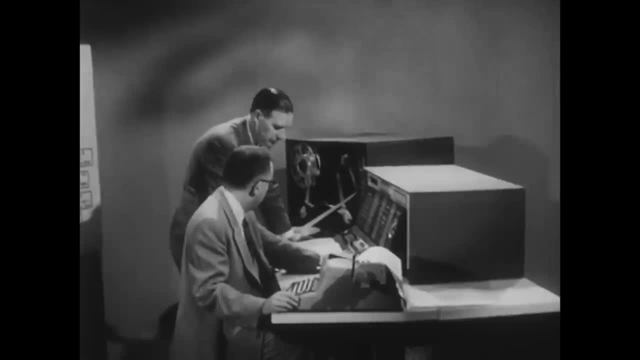 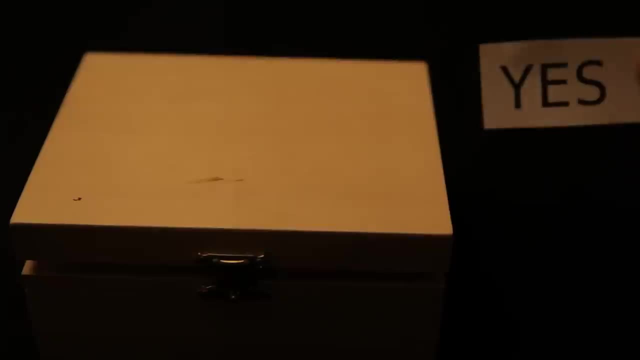 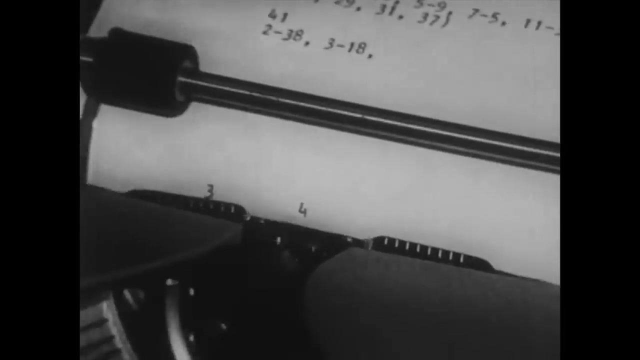 to think about the possibility of the mechanical process, that is, automatic machines which could answer questions. For example, one of his challenges was a machine which could answer yes or no as to whether a given statement about mathematics is true, If such a mechanical process existed. 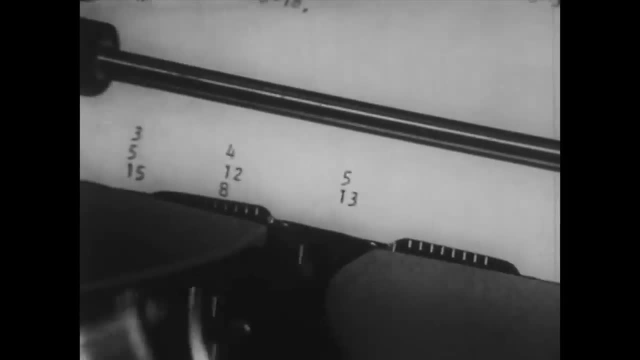 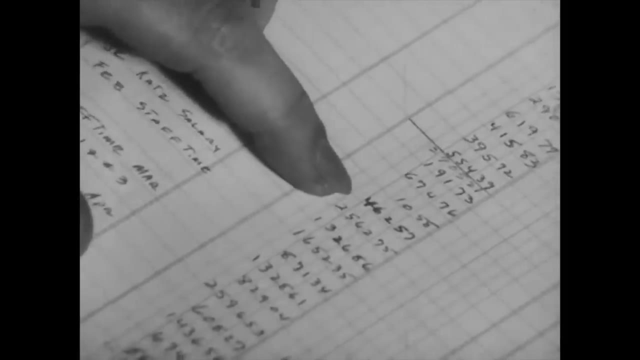 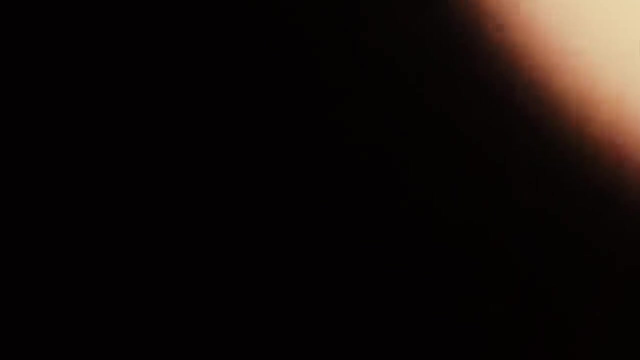 it would completely automate the work of all mathematicians, And at the time, calculation machines were well known, of course, but thinking machines were not, And so the mechanisms of these decision machines weren't yet defined. People were still speculating, And this is where Alan Turing enters the story. 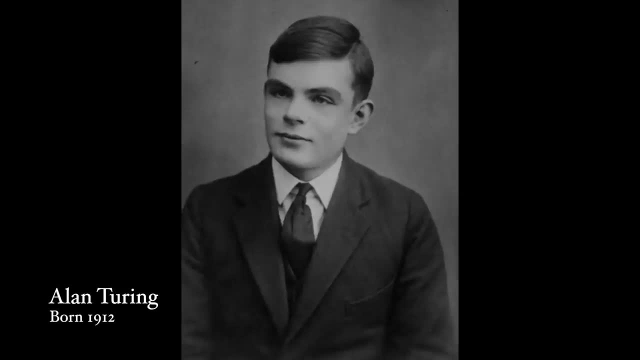 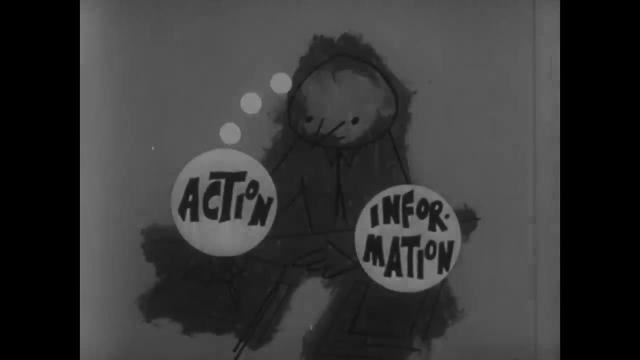 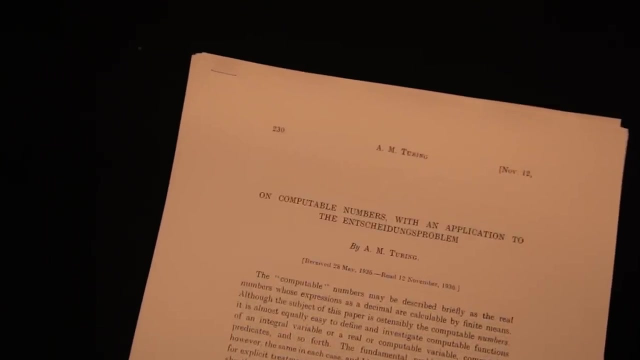 Since childhood, he was fascinated with the complex mechanisms behind the human mind. Since childhood, he was fascinated with the complex mechanisms behind the human mind. Turing simplified everyone's conceptions of what physical form these decision machines would actually take, And in 1928, he published a historic paper. 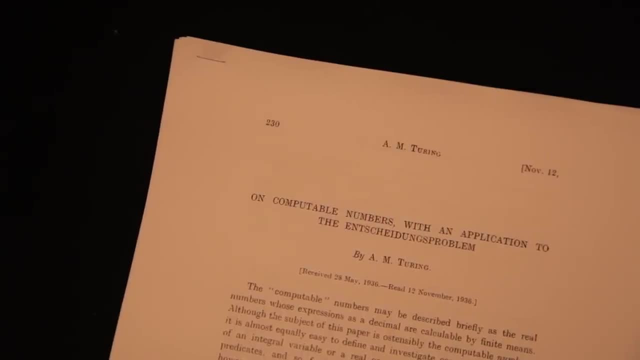 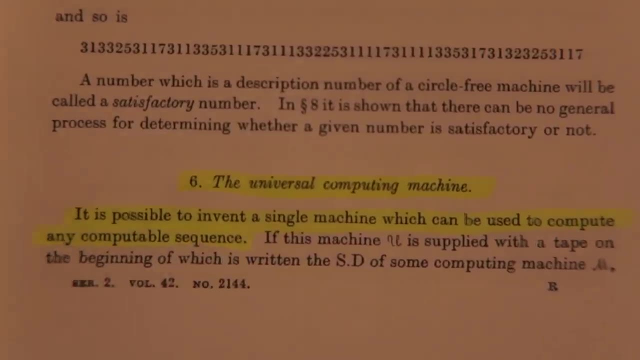 that directly addressed Hilbert's challenges. In it he imagines a machine that can do anything any other machine might do, known as a universal machine, And he begins by imagining a machine as a human in a box with a machine that can do anything any other machine might do. 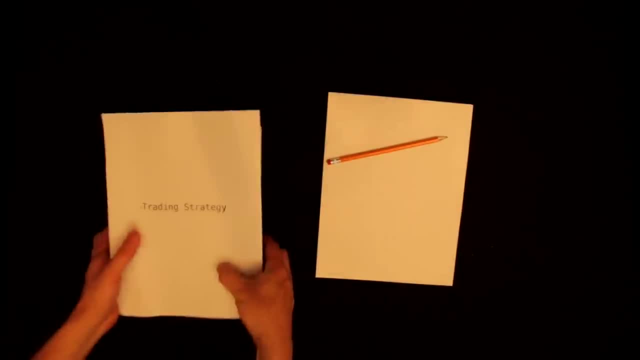 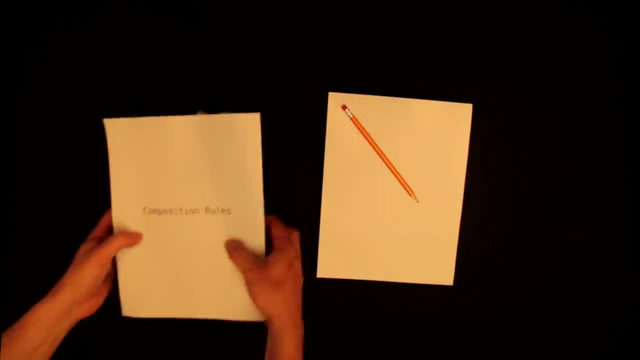 And he begins by imagining a machine as a human in a box with a machine that can do anything any other machine might do- a pencil and a stack of paper- and they are handed a book of instructions to follow. So in order to change what this human does, you must alter the instructions in the book. 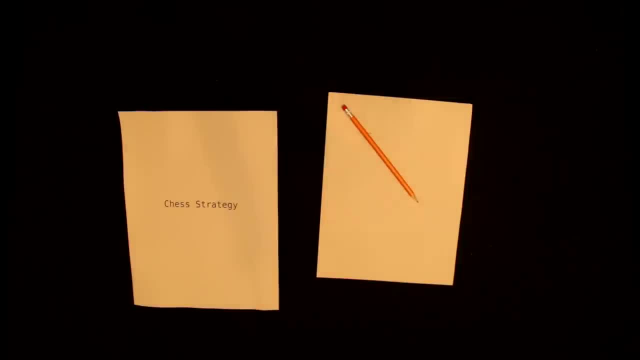 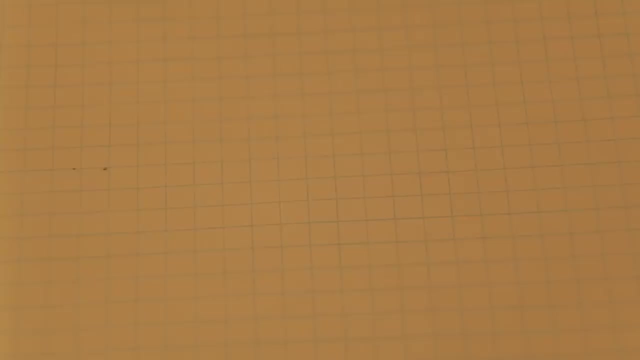 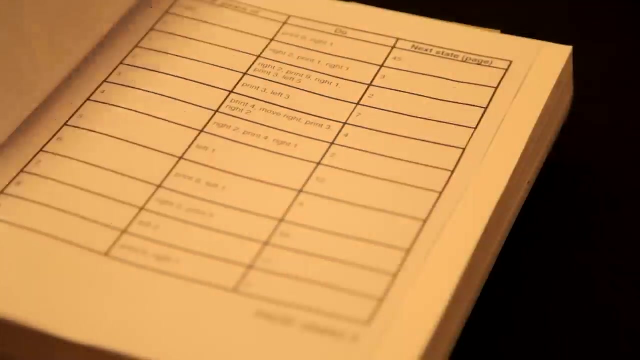 That's the deep insight he had: defining behaviour with symbols instead of mechanisms. This was a very clever trick at the time, so he spends the first 60% of his paper laying out precisely how it would work and what form these written instructions or algorithms would take, as follows. 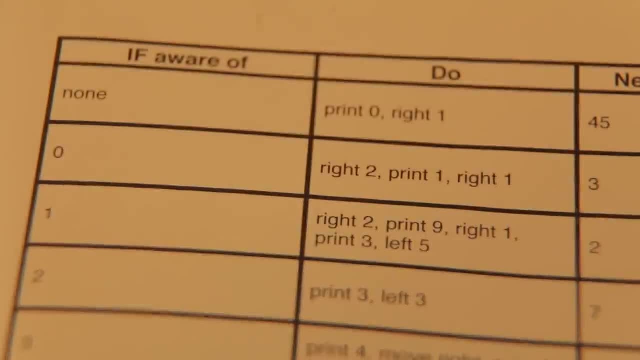 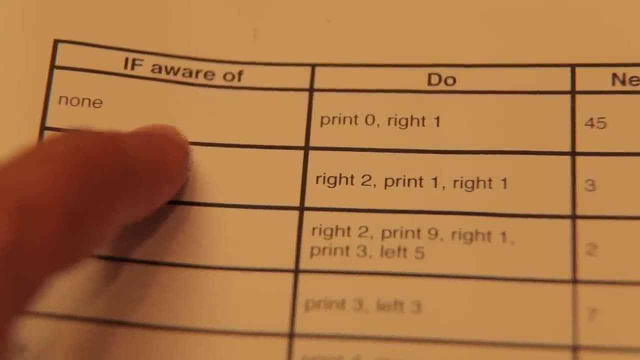 Think of each page in this book of instructions as a single decision. First comes an observation, which is the if-half of the conditional statement, and what the person is doing. What the person is observing is precisely where their pencil is pointing in the rough work. 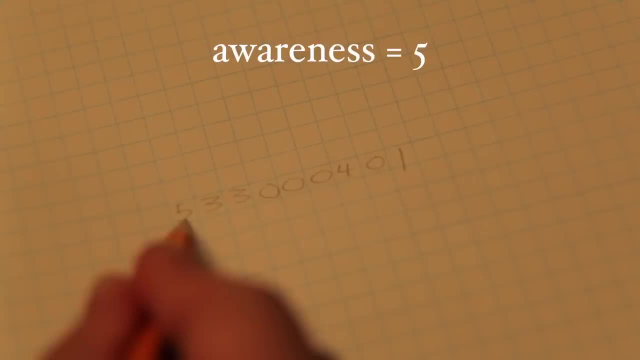 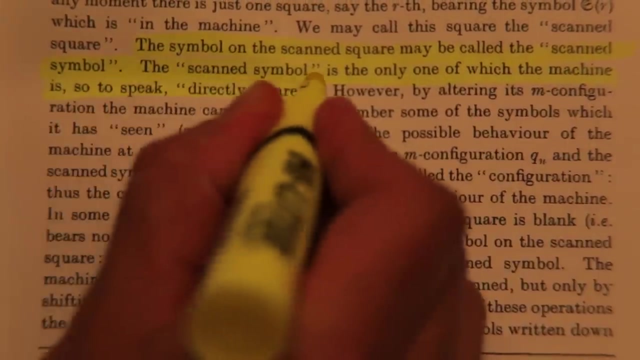 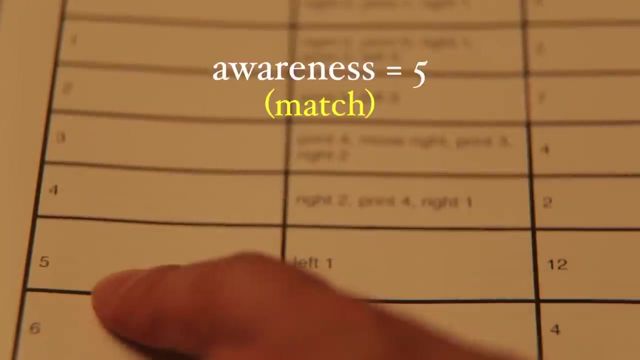 In our example it's the first symbol of the input. He calls this their awareness. so they are only ever aware of one symbol. Next they look at their instructions and compare the symbol in their memory to a list of possibilities in the first column to find a match. 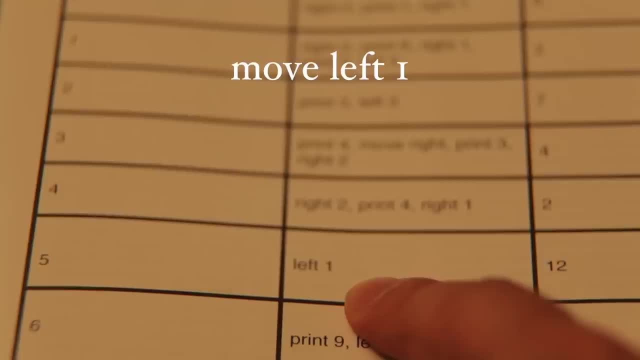 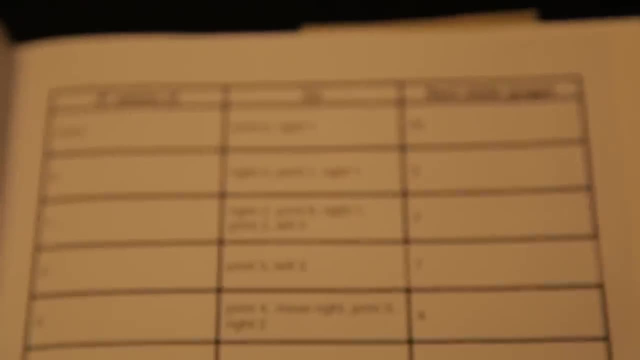 Once a match is found, they move on to the second symbol, the next step of the conditional statement, the operation step. And what they do here is interesting. Turing observes that, no matter what the instructions are or what language they are in, they are only ever going to be writing down symbols on the paper. 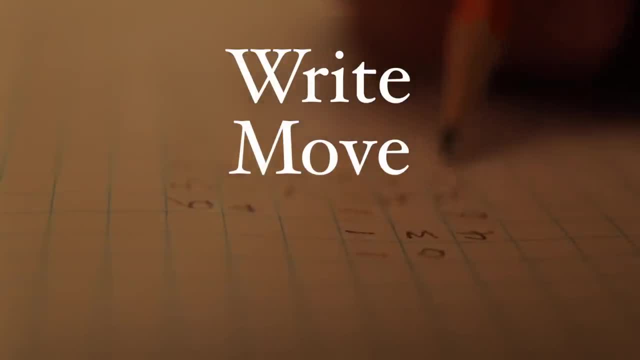 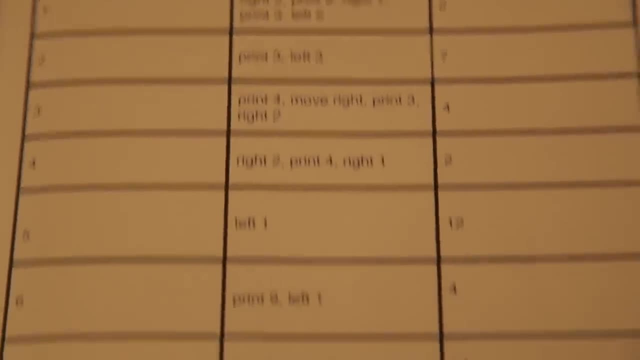 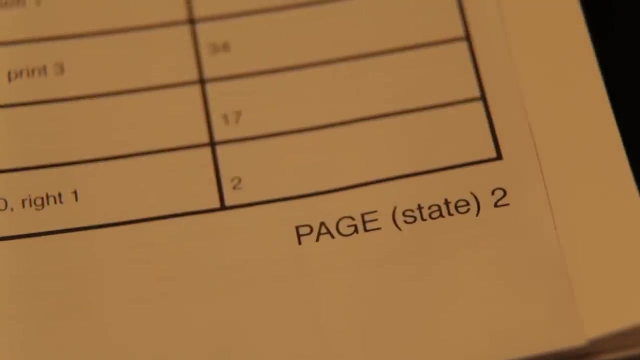 and or moving their attention to some new location. And so the last column in the table, called next state, lists the next page to jump to In this book. analogy: each page in the book is a new step. Turing calls these steps states of the machine. 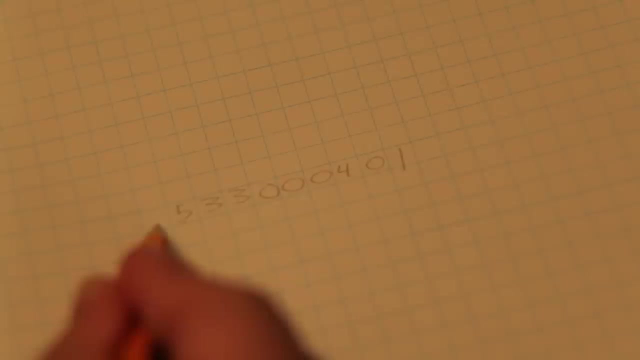 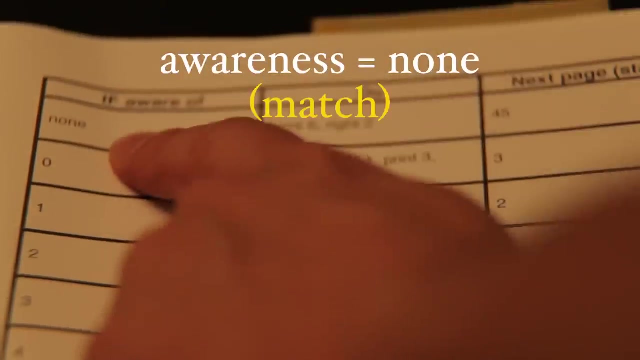 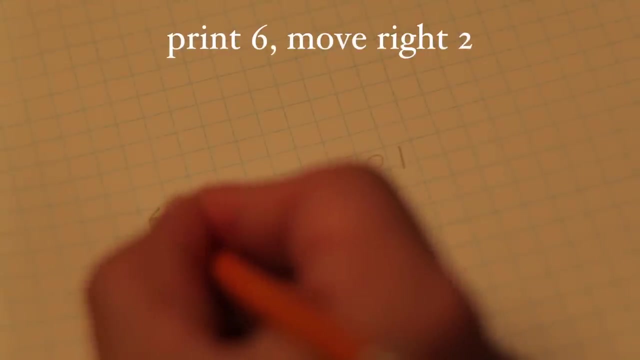 And when the next state is arrived at, their current awareness where their pencil is currently pointing is observed again, And then they scan to find a match in the same way. Once they do, they follow the sequence And then jump to the next state. 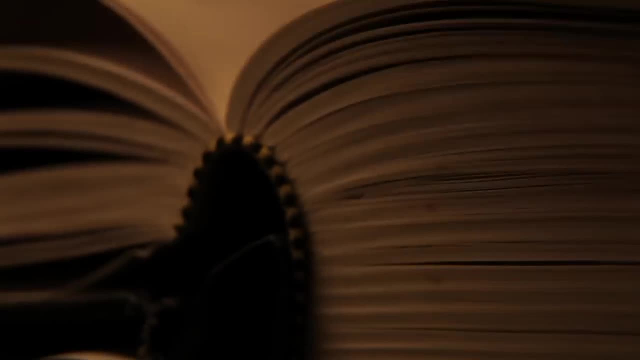 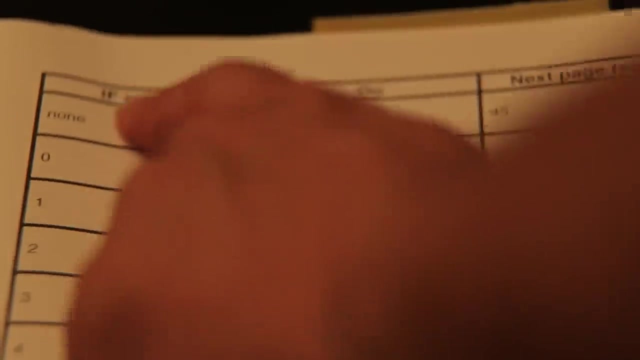 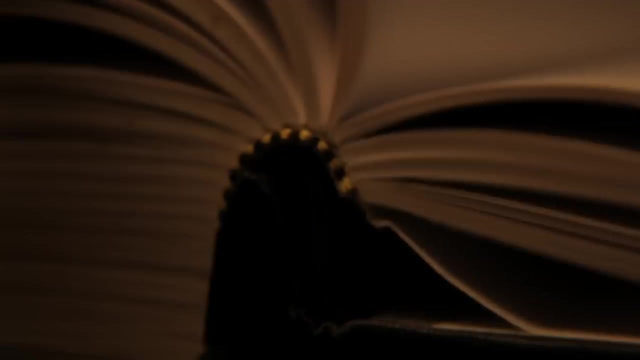 And this process continues state after state. And so the process of computation is exactly like turning pages in a book and, at each page, making a decision about what to do next, based on where the pencil is pointing on a separate page- And note that this book wouldn't be read in the same linear order. 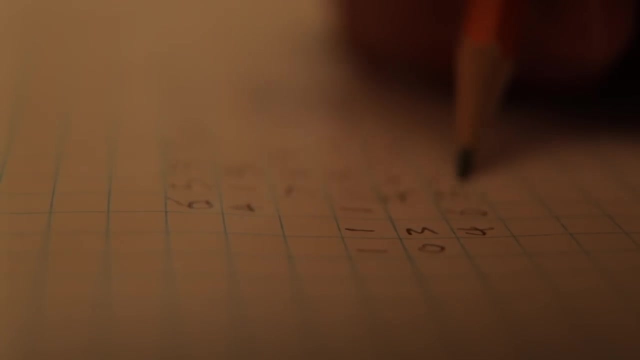 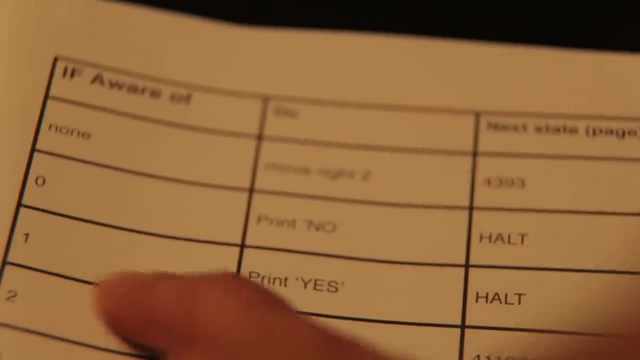 It's more like a choose-your-own-adventure at each page, because the sequence in which they flow through the pages or states will depend on the input they receive. But eventually this process leads to a final state where they write down an answer. 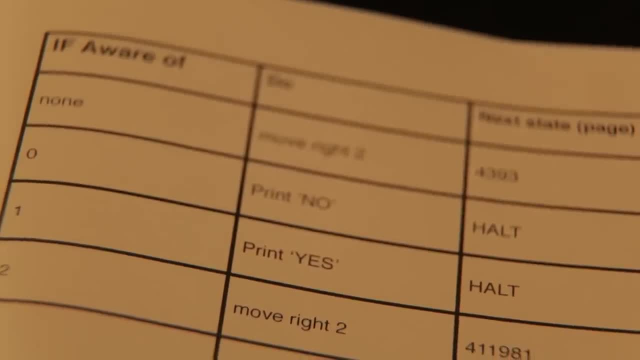 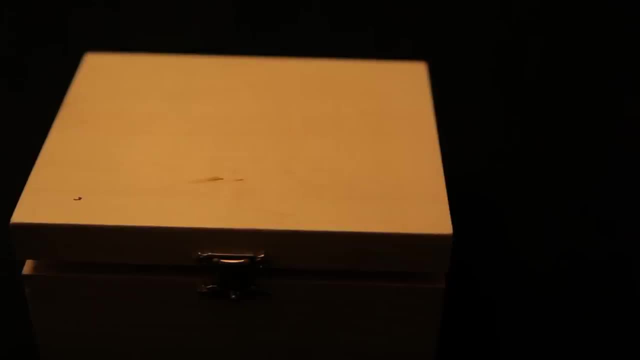 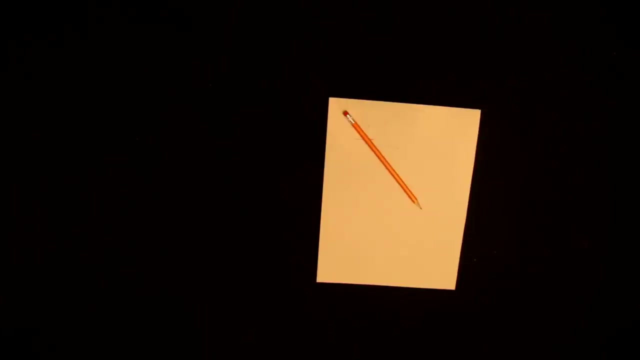 and halt or stop, And they output their result. And that's how it works. Notice, the decision-making power of this machine is stripped away from the human. All of the logic of their behavior is based on how the book, or algorithm, is designed. 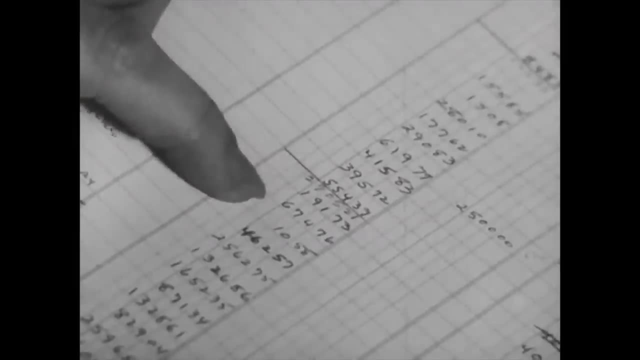 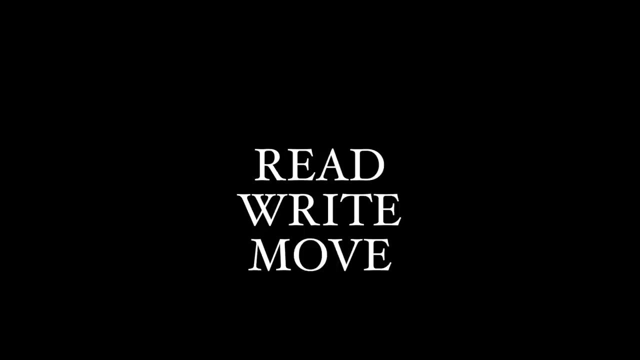 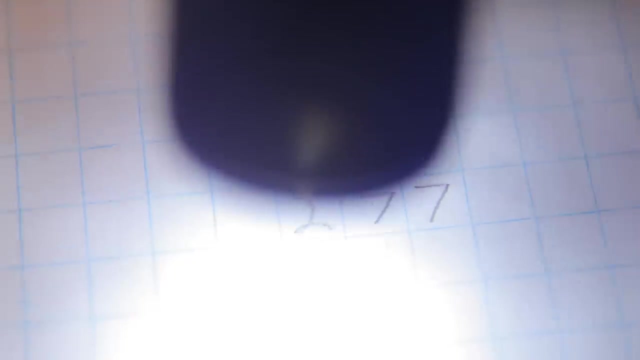 What we call the program, And Turing notes that all of these steps could be done with pre-existing technology. We don't need a human As follows, For reading symbols off the paper. Turing imagines a simple scanner head which can move around and read individual symbols. 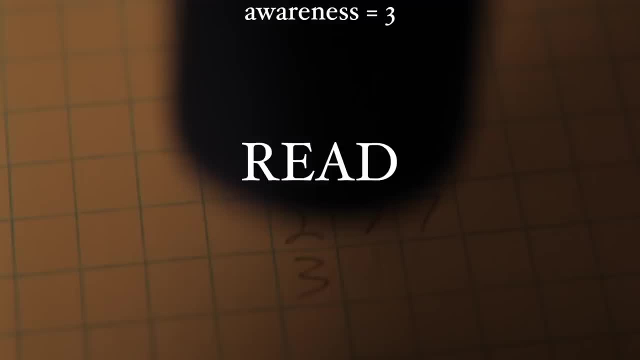 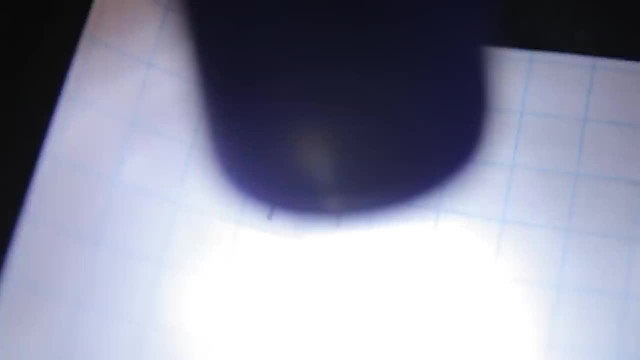 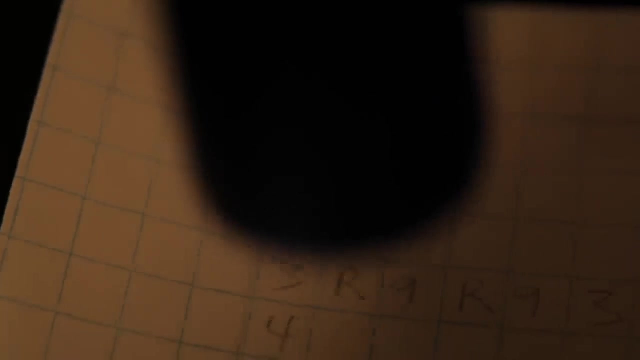 one at a time into some form of memory known as a read operation, And then it would move to the current state and identify when a value in the first column matches the scanned symbol, And once a match is found, it moves over to the operation step. 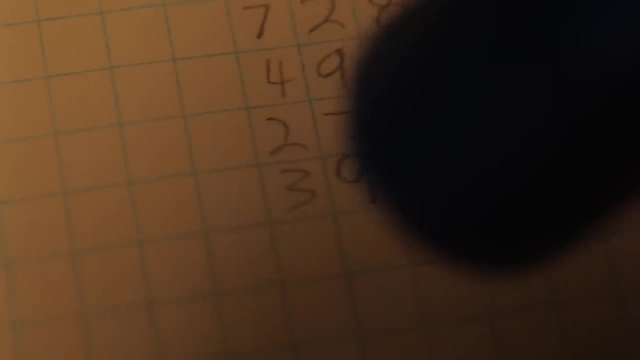 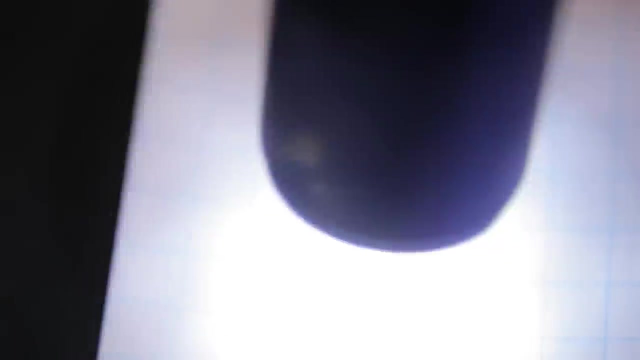 And lastly, it also contains a printer which can output symbols given by the instructions known as print operations, And that's all it does: Read, move, print Over, and, over and over again. And to further simplify this, Turing reminds us that the book you provide 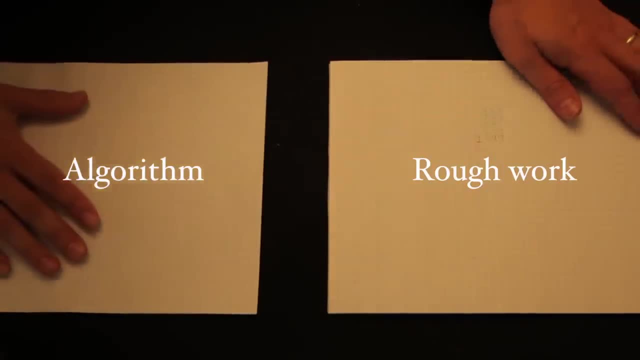 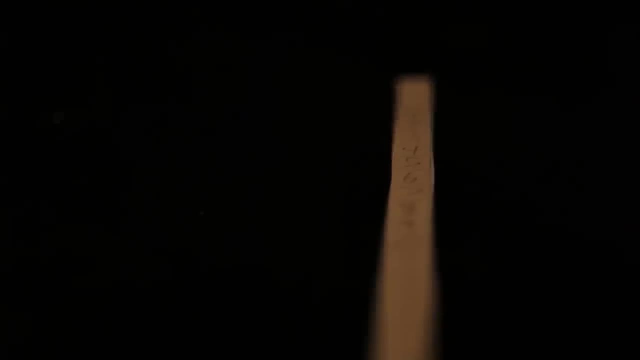 or the algorithm and the rough work could all be done on one big piece of paper, And that paper could be arranged in a long array instead of a 2D sheet, Leading to his famous simplification of a machine which is essentially a roll of tape. 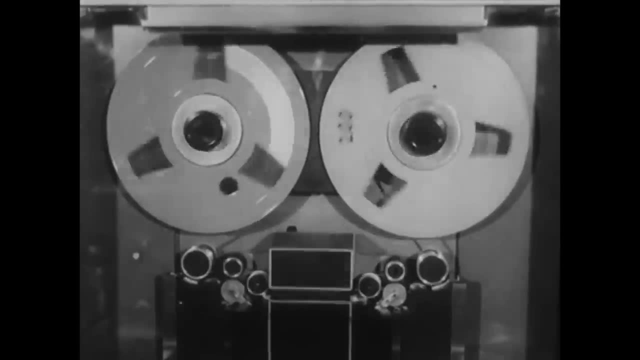 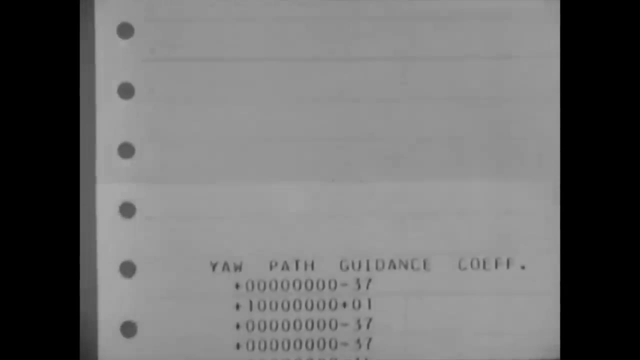 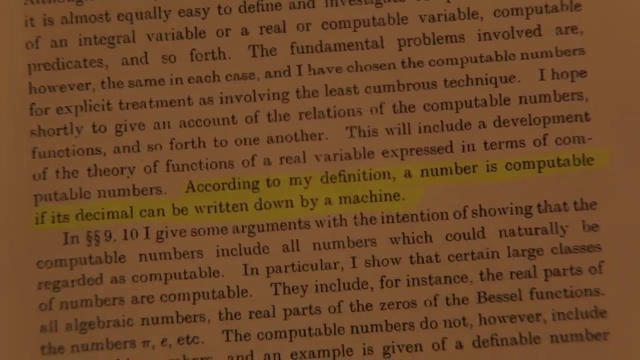 and a scanner printer head, And any symbolic process performed by a modern computer can be performed by this simple machine. Turing states that anything his universal machine can write down is what we call computable. So a computable problem is a problem that a Turing machine could be programmed to solve. 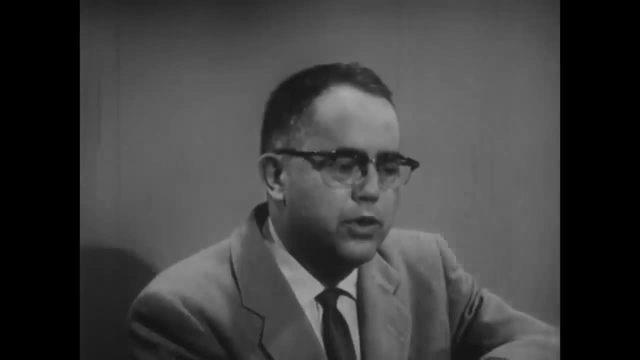 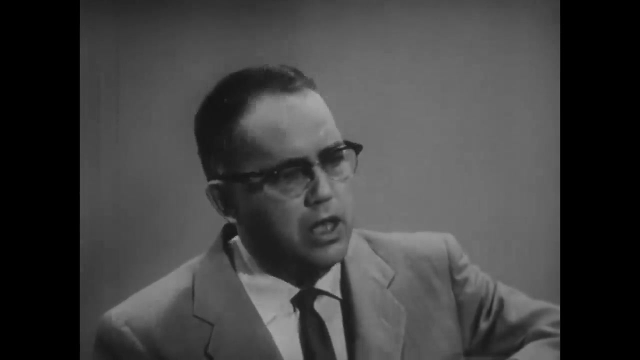 given enough time and space to do it. A computer, as we know it today, is a device which can accept information in some form, store it, process it and produce answers in an acceptable, readable form. With this definition, of course, goes the injunction. 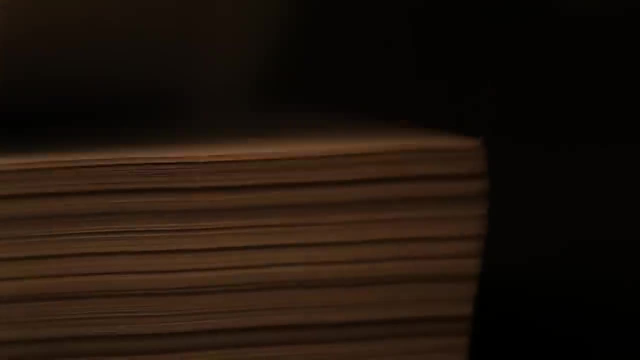 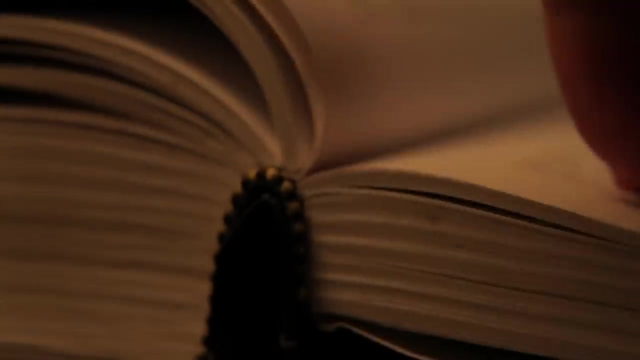 if we're going to call it a computer, that it must be able also to store its own instructions and process them from within the machine. And so Turing showed that all the power of machines, or the future computers, would be based on how you designed the instruction table.